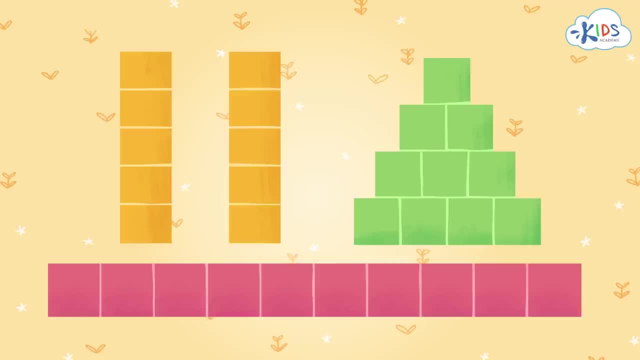 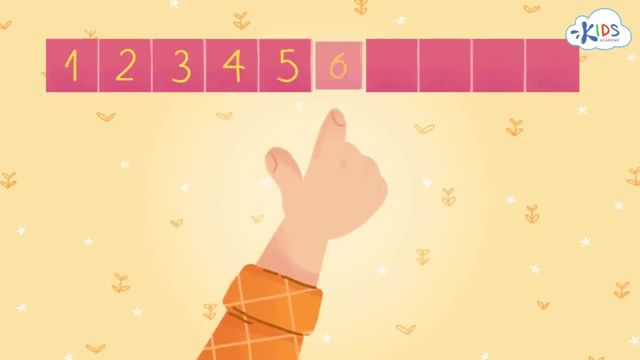 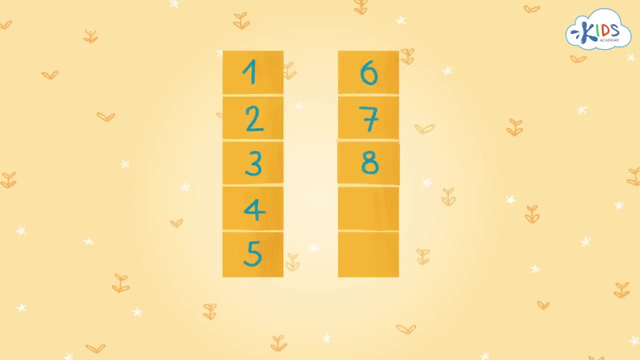 shape. we can count and see that they each have 10 blocks: 1,, 2,, 3,, 4,, 5,, 6,, 7,, 8,, 9,, 10.. There are 10 red blocks in a line. Do you think there are 10 orange blocks too? Let's count them: 1,, 2,, 3,, 4,, 5,, 6,, 7,, 8,, 9, and 10.. The orange blocks were in two groups with five blocks each, just like the fingers on your hands. One hand has five fingers and two hands makes 10.. 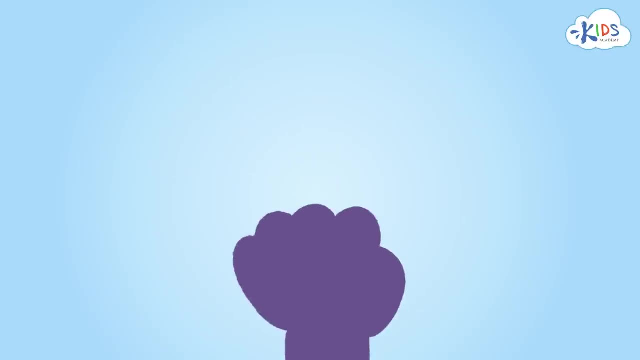 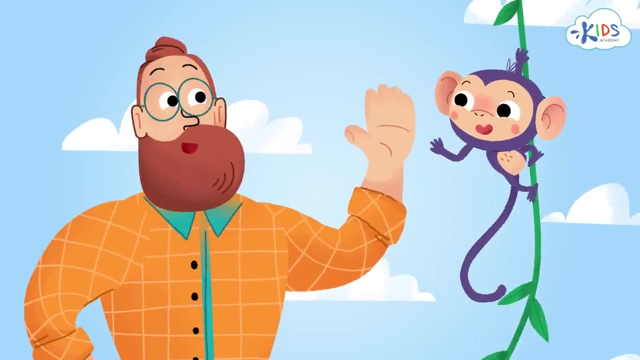 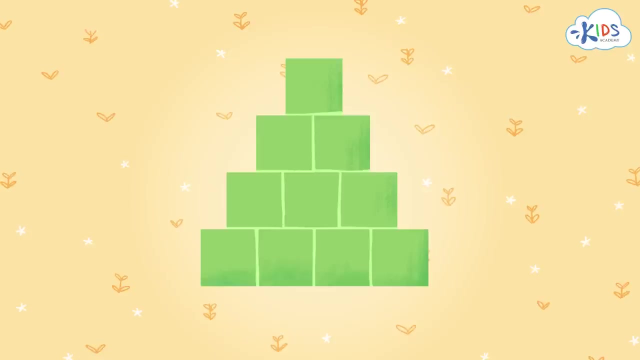 Hey, look that monkey has five fingers too: 1,, 2,, 3,, 4,, 5,. give me 5, a little buddy. Look at this group. do you think there are 10 green blocks in this pyramid? Let's. 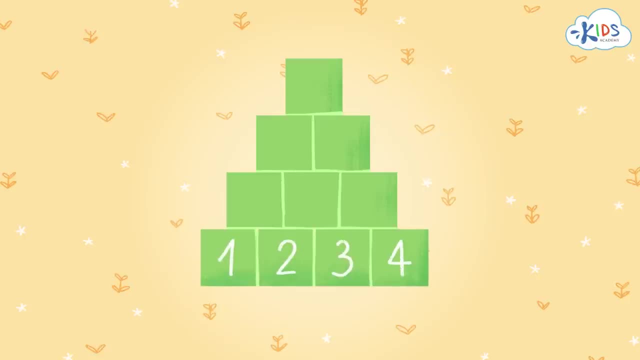 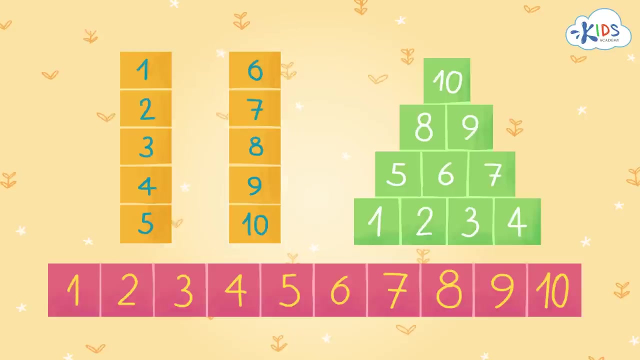 count and see: 1,, 2,, 3,, 4,, 5,, 6,, 7,, 8,, 9,, 10!. Yes, this group has 10 too. Sometimes can find 10 by seeing one of these patterns. Which group was easiest for you to count? 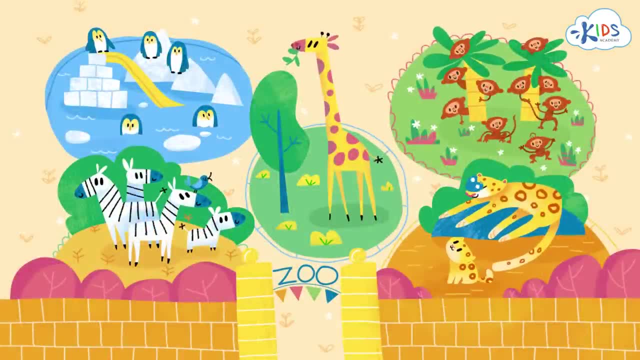 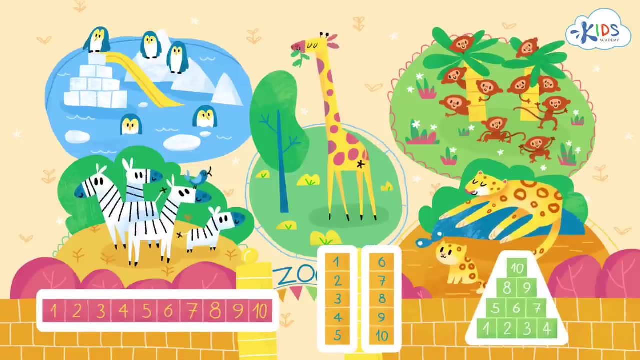 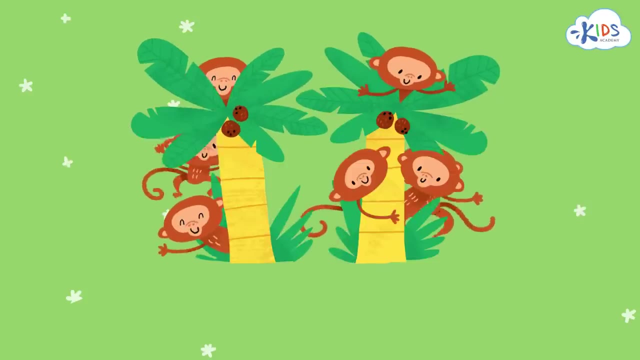 Okay, boys and girls, now it's time to find the groups of 10 animals in the zoo. Let's use these groups to help us count and find 10. with other things too. Whoa, Look, Now that's a lot of monkeys. I wonder if there are 10. If we move them around? 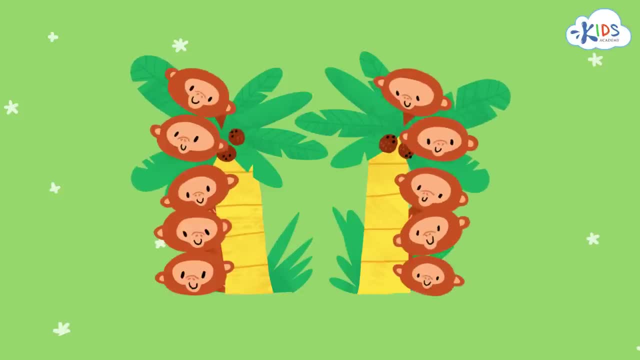 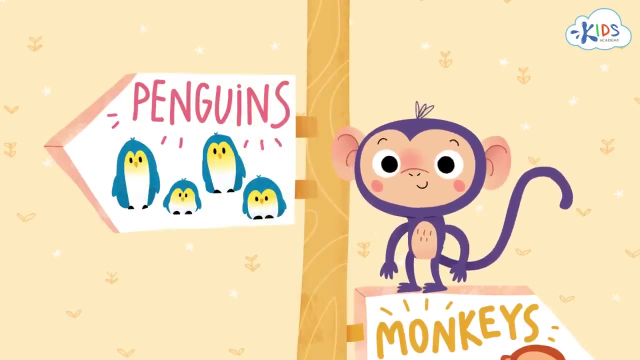 and try to put them into two equal rows. are there five in each row? Yes, Look, Five and five make 10.. It looks like this pattern. Our monkey friend wants us to go see the penguins. It's your turn. Let's go to the penguin pool and see if you can find groups of 10.. 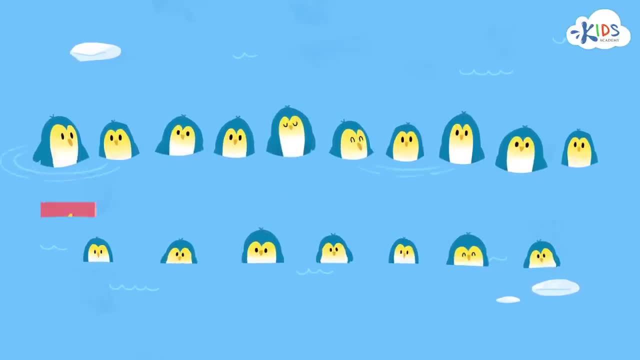 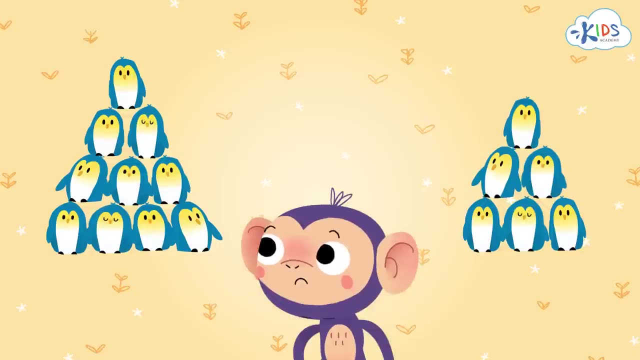 Do you see which one has 10? It's this one. Do these groups show 10 penguins? Now, that's a tough one. I see two pyramids, but do they both show 10? Nope, We always count to check: One, two, three, four, five, six. 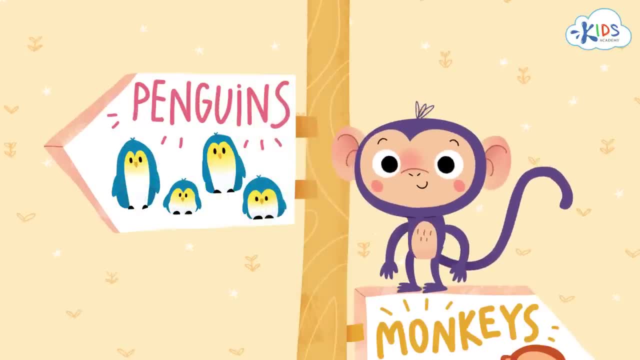 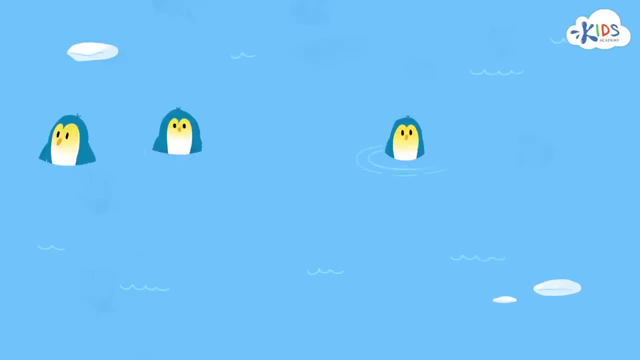 Our monkey friend wants us to go see the penguins. It's your turn. Let's go to the penguin pool and see if you can find groups of 10.. Do you see which one has 10? It's this one. Do these groups show 10 penguins? 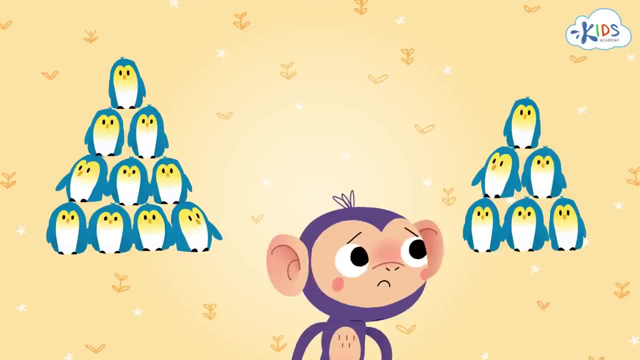 Now, that's a tough one. I see two pyramids, but do they both show 10?? Nope, We always count to check: One, two, three, four, five, six. One, two, three, four, five, six. 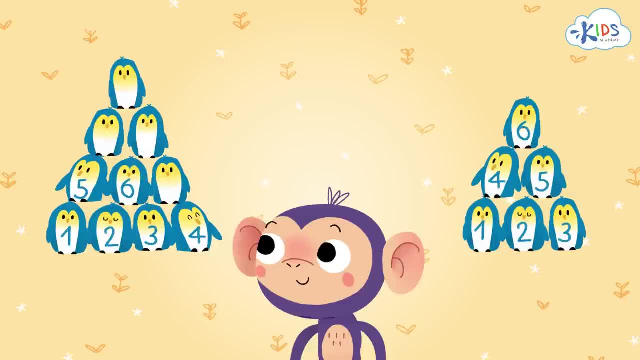 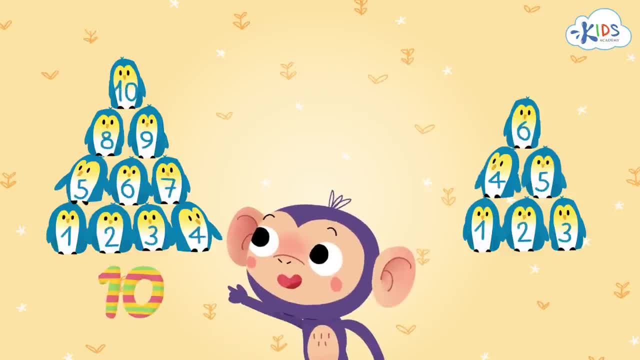 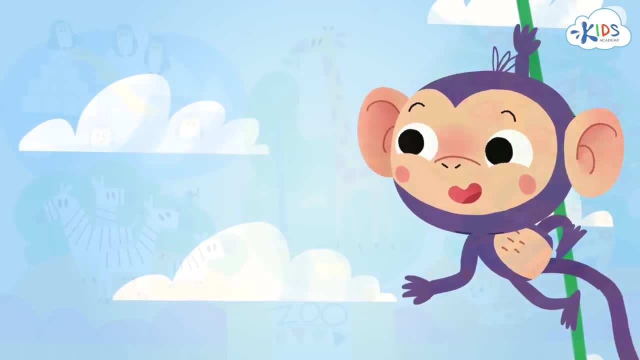 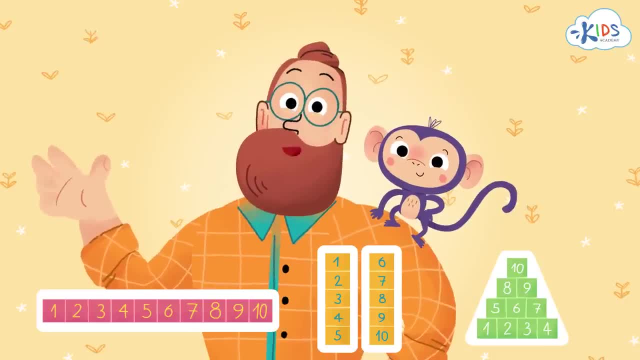 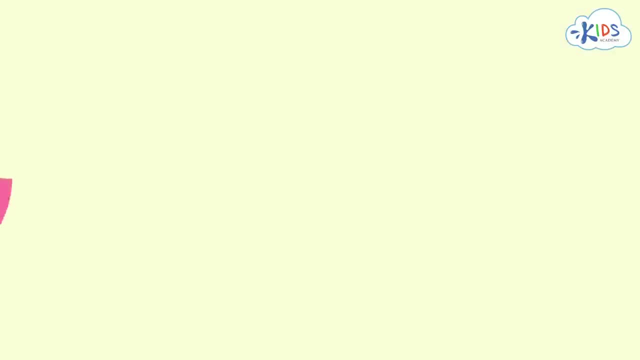 It looks like this is the group that shows 10.. It looks like this is the group that shows 10.. groups of 10.. See you next time, When we look at a number like 35,. each digit in this number has its own value. 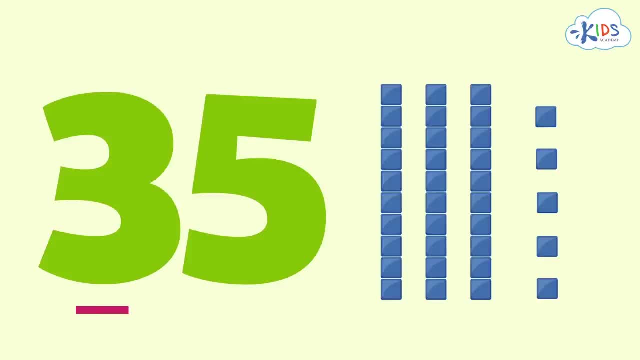 There is a number in the ones place and a number in the tens place. Let's have a closer look at each number to see its true value. The ones place is furthest to the right. The number in the ones place always equals itself In our number 35,. 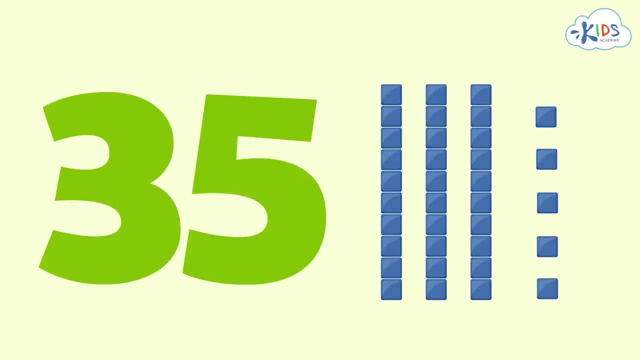 the 5 is in the ones place. Its value is just that, 5. It is represented by the five ones cubes. The next place over is the tens place. The number in the tens place is always 10 times the value the number shown. It's like counting by tens. 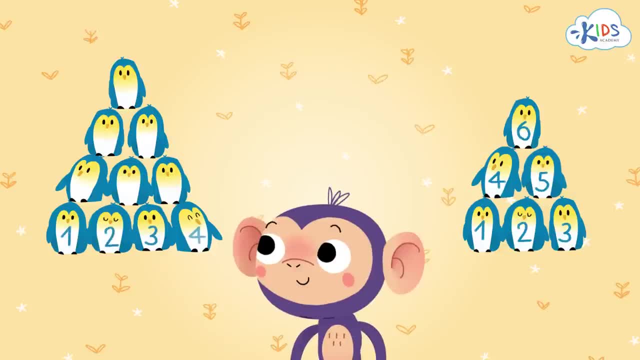 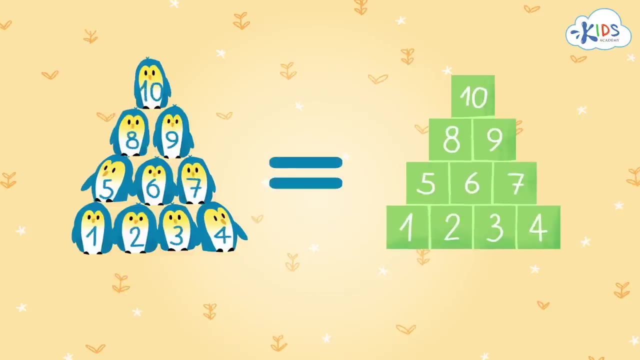 One, two, three, four, five, six, Two, three, four, five, six, seven, eight, nine, ten. It looks like. this is the group that shows 10.. 10- It looks like this: 3,, 2,, 3, 4.. 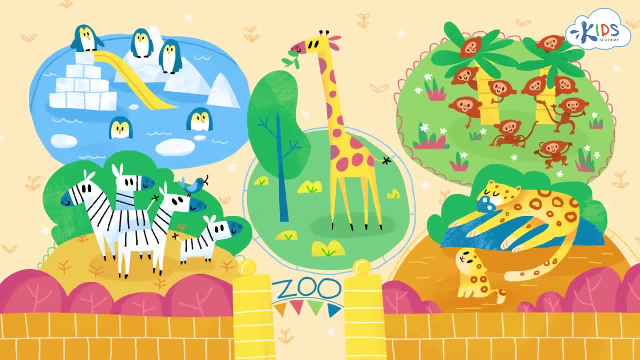 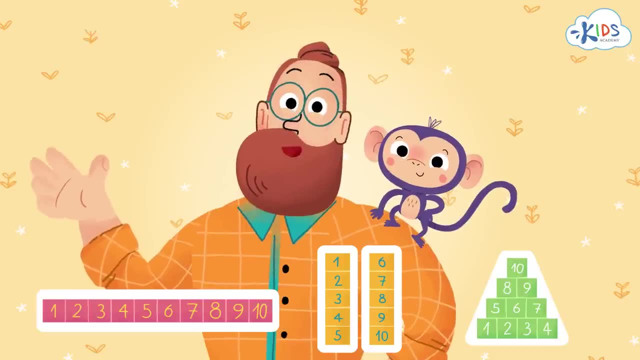 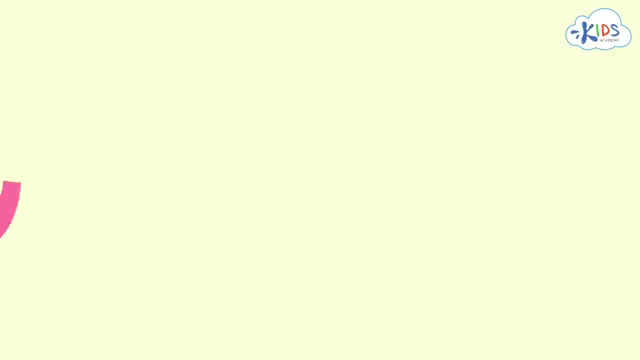 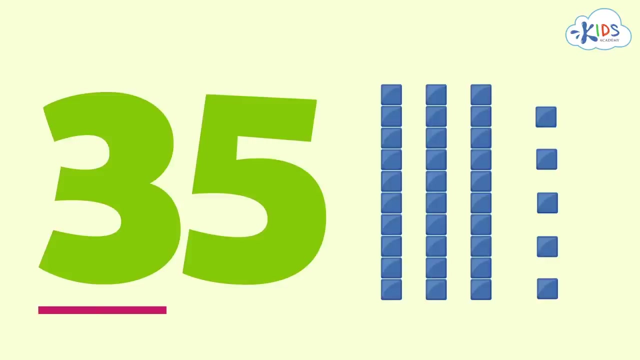 Podcast challenge 10 encore. Thanks for watching boys and girls And thanks for helping me count, look for patterns and count groups of 10.. next time when we look at a number like 35, each digit in this number has its own value. there is a number in the ones place and a number in the tens place. 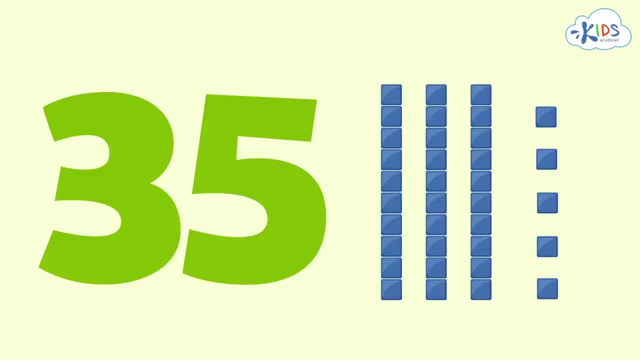 let's have a closer look at each number to see its true value. the ones place is furthest to the right. the number in the ones place always equals itself. in our number 35, the 5 is in the ones place. its value is just that: 5. it is represented. 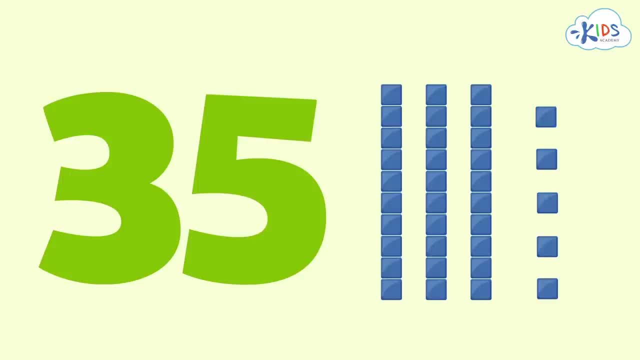 by the 5 ones cubes. the next place over is the tens place. the number in the tens place is always 10 times the value the number shown. it's like counting by tens to the number. you see in our number 35 the 3 is in the tens place we can find: 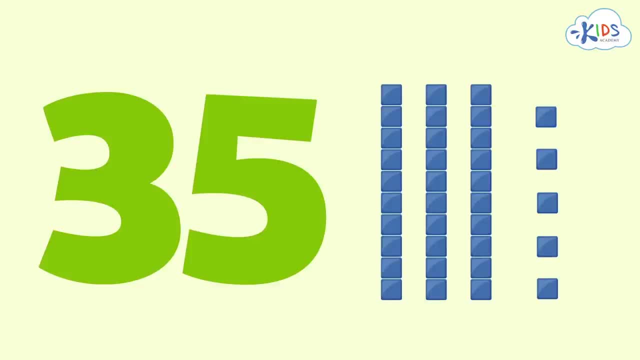 its value by counting by tens 3 times. let's try it: 10, 20, 30. the value of the 3 is 30. another trick you can remember is to just put a 0 at the end of the number. the 3 in 35 is represented by the. 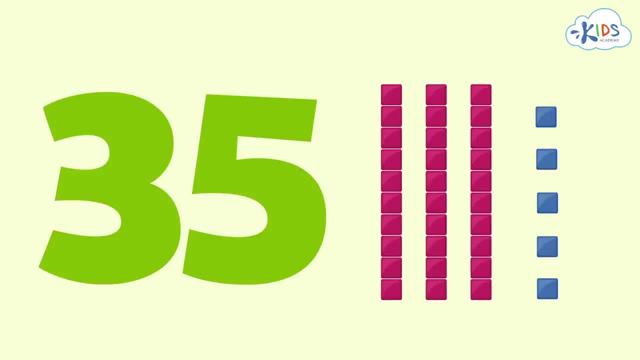 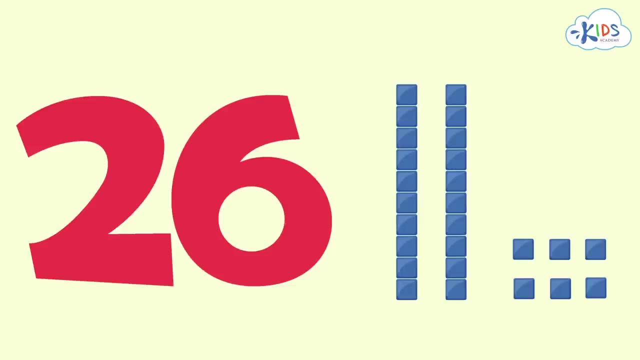 3 tens blocks, which equals 30. in the number 26, the 6 is in the ones place and the 2 is in the tens place. the 6 is worth just 6, which is represented by 6 cubes. the 2 is worth 20 because it is in the tens place and is represented by the. 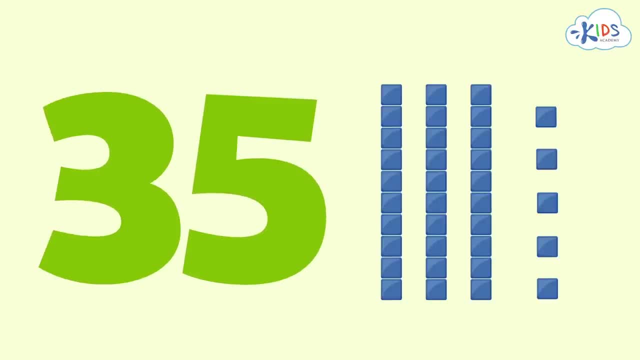 to the number you see In our number 35,. the 3 is in the tens place. We can find its value by counting by tens three times. Let's try it: 10,, 20, 30. The value of the 3 is 30. Another. 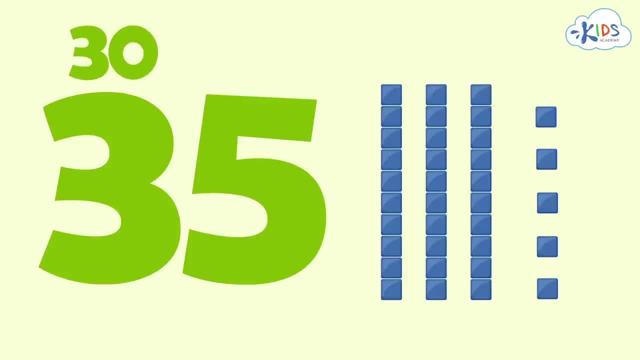 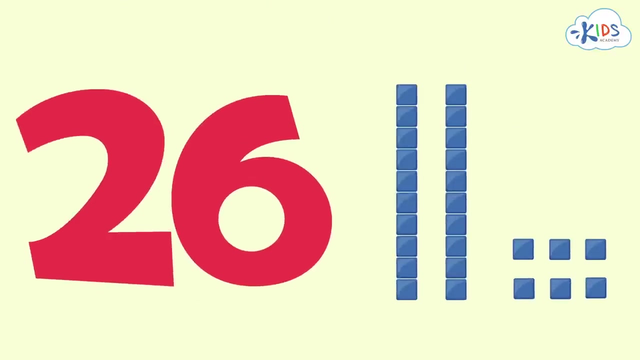 trick you can remember is to just put a zero at the end of the number. The 3 in 35 is represented by the three tens block, which equals 30. In the number 26,, the 6 is in the ones place and the 2 is in the. 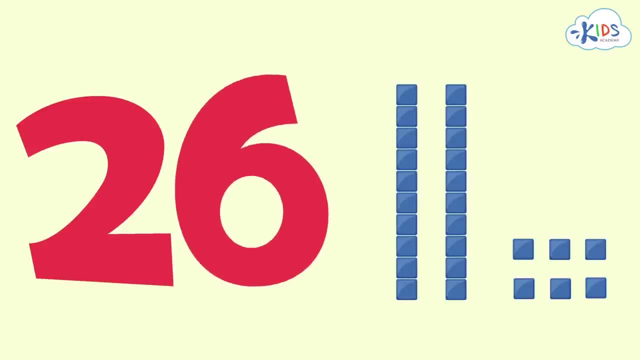 tens place. The 6 is worth just six, which is represented by six cubes. The 2 is worth 20 because it is in the tens place and it is represented by the two long tens blocks. You can count by tens using the base 10 blocks or just count in your. 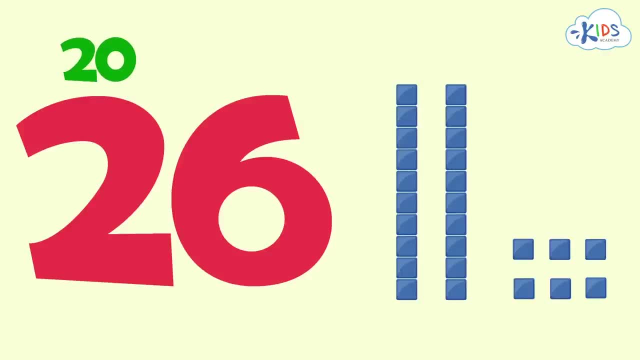 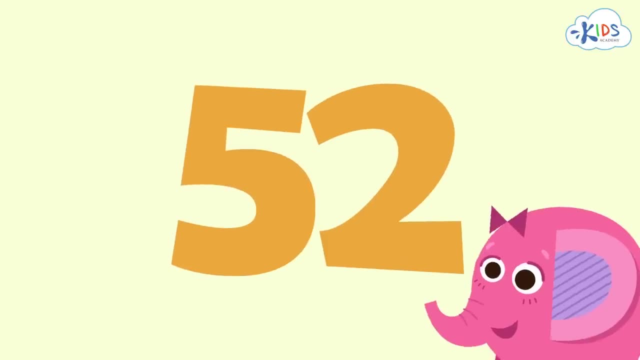 Can you tell the value of the digits in the number 52?? What is the value of the five? What is the value of the two? I'll give you some time to think, but if you need more time, you can pause the video and answer when you're ready. 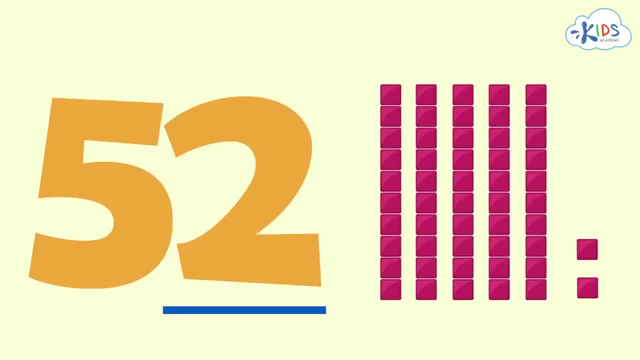 Okay, here's the answer. The two is in the ones place, so it's just worth two. The five is in the tens place, so we'll have to count by tens, five times 10,, 20,, 30,, 40,, 50.. 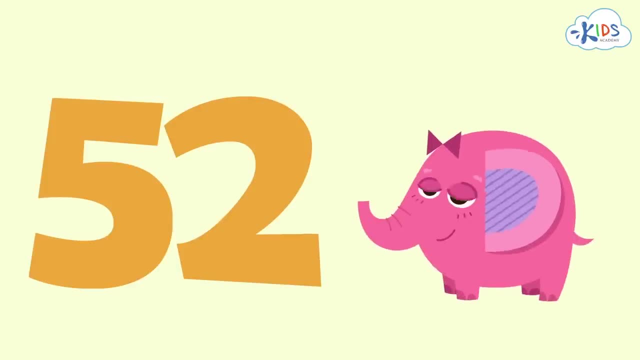 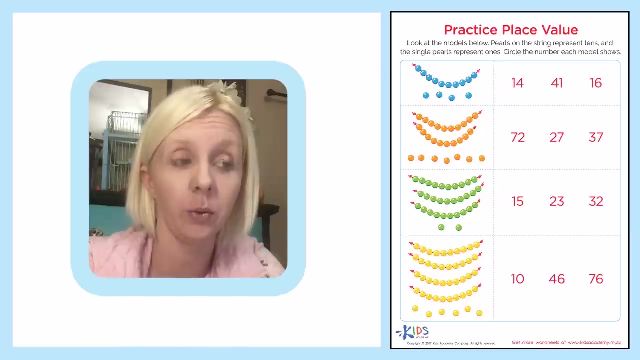 The value of the five is 50.. Remember to look at the place the digit is in before you decide the value of that number. Thanks for watching boys and girls. See you next time. Okay, so we have practice to make all the numbers in the place value. 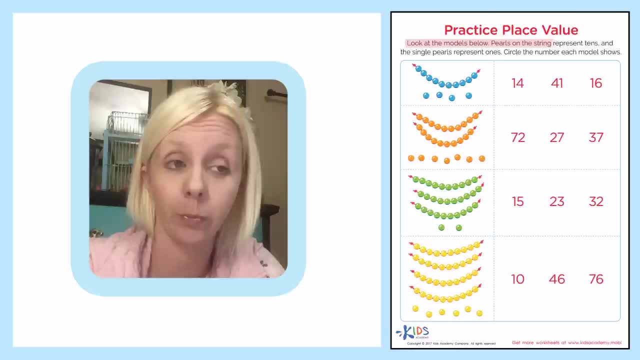 And the directions say: look at the models below. Pearls on the string represent tens and the single pearls represent ones Circle the number each model shows. So we can do this a couple of different ways. The first way that I'm gonna show you: 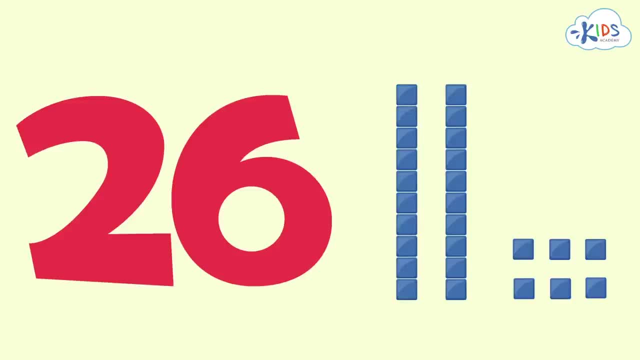 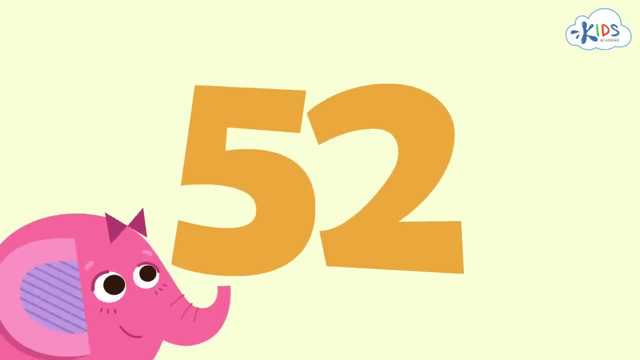 2 long tens blocks. you can count by tens using the base 10 blocks or just count 10, 20. I'll leave you with a challenge. can you tell the value of the digits in the number 52? what is the value of the 5? what is the value of the 2? I'll give you. 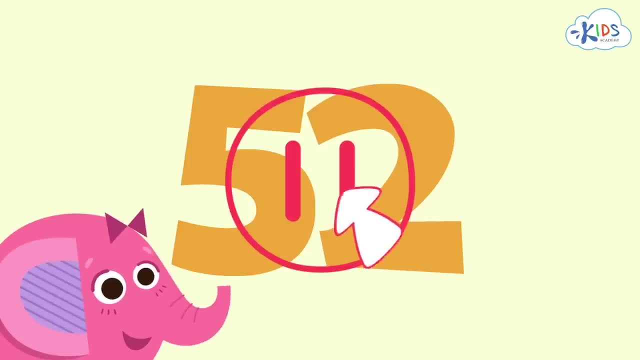 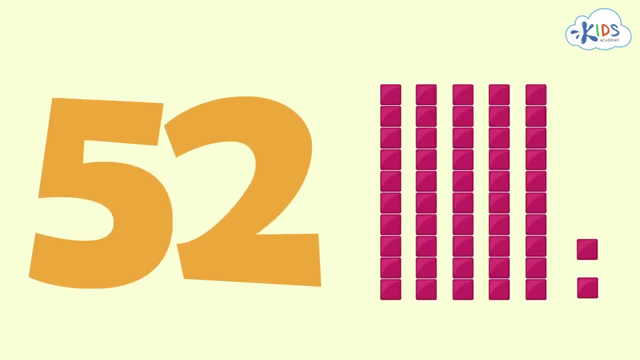 some time to think, but if you need more time, you can pause the video and answer when you're ready. okay, here's the answer. the 2 is in the ones place, so it's just worth 2. the 5 is in the tens place, so we'll have to count by tens, 5 times 10, 20, 30, 40, 50. the value of the 5 is 50. 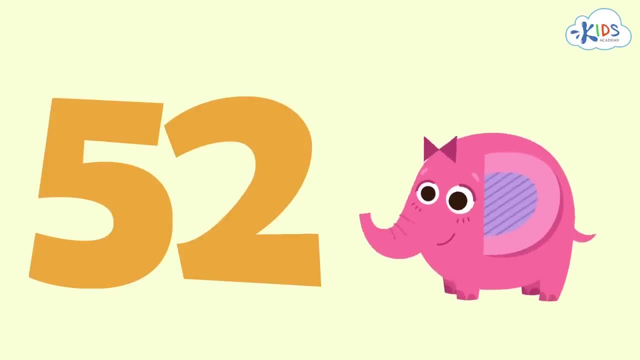 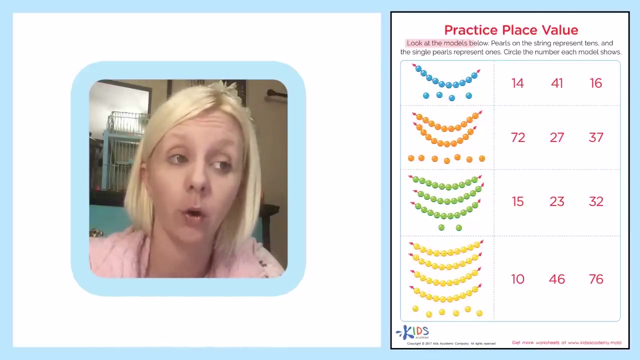 remember to look at the place the digit is in before you decide the value of that number. thanks for watching boys and girls. see you next time. okay, so we have practice place value and the directions say: look at the models below. pearls on the string represent tens and the single pearls represent ones circle, the number each. 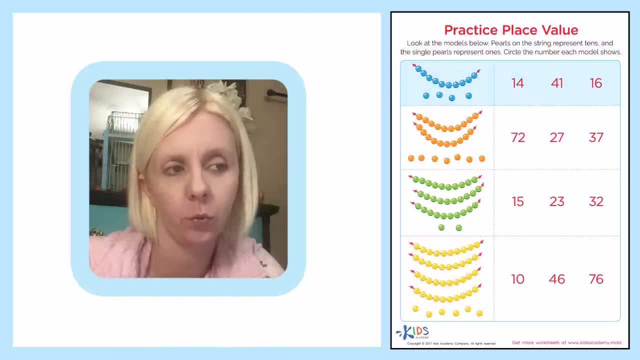 model shows. so we can do this a couple of different ways. the first way that I'm going to show you is just to count by tens and ones. so one way that you can do it is you can count how many pearls on a string there are. so this is going to be. 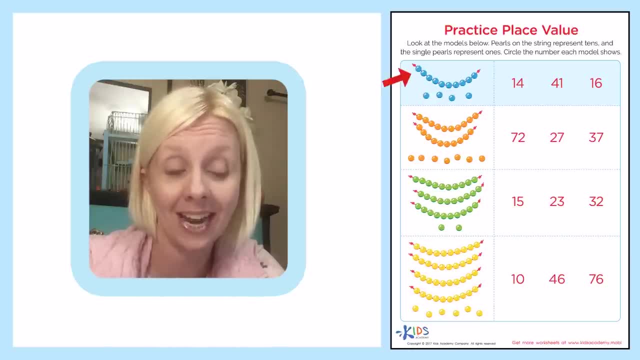 tens and you're going to count by tens, so there's only one, first of the sevenINK. so we're going to go 10 and then we're going to count up 11, 12, 13, 14. that's one way to come up with the number and the number is 14. 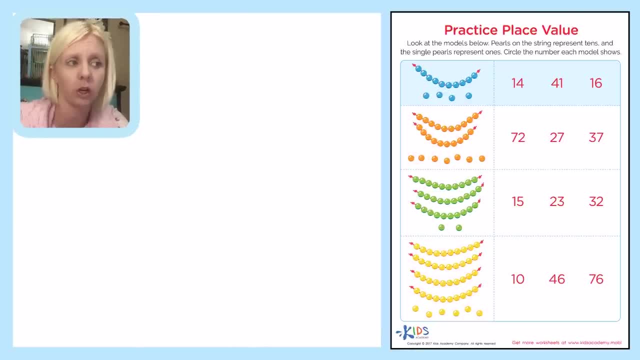 right over here. another way that you can do it- and I look kind of like this way, because I like to keep everything organized- is to make a t chart, and a t chart is basically like a lowercase T, but what we're gonna do is we're gonna 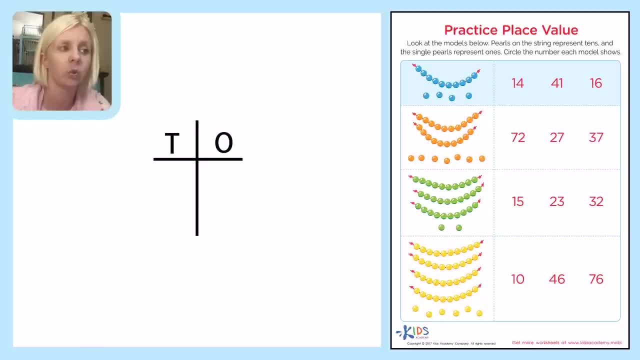 put tens on the left side and ones on the right side. so let's count how many strings of 10- we have just one, so we're going to put a one over here- and how many individual or single pearls do we have. we have one, two, three, four, so you can count those up and write it up and you 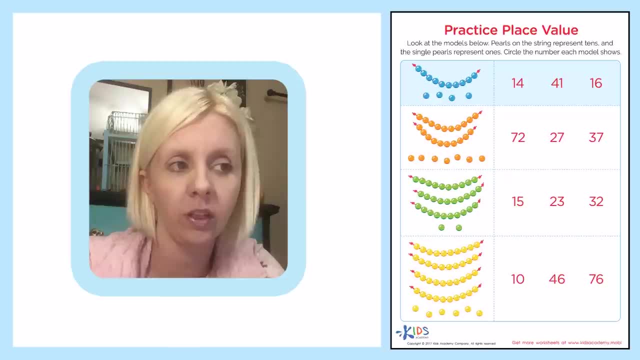 is just to count by tens and ones. So one way that you can do it is you can count how many pearls on a string there are. So this is gonna be tens and you're gonna count by tens. So there's only one tens. 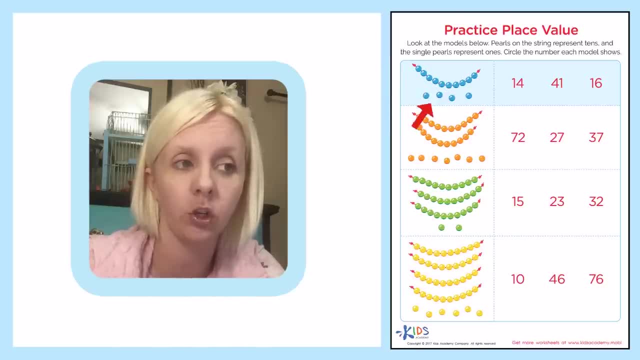 so we're going to go 10, and then we're going to count up 11,, 12,, 13,, 14.. That's one way to come up with a number, and the number is 14 right over here. Another way that you can do it, and I kind 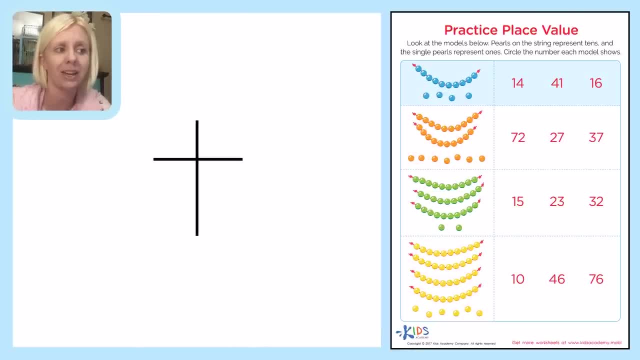 of like this way- because I like to keep everything organized- is to make a t-chart, And a t-chart is basically like a lowercase t, but what we're going to do is we're going to put 10s on the left side and ones on the right side, So let's count how many strings we have of 10.. We have just one. 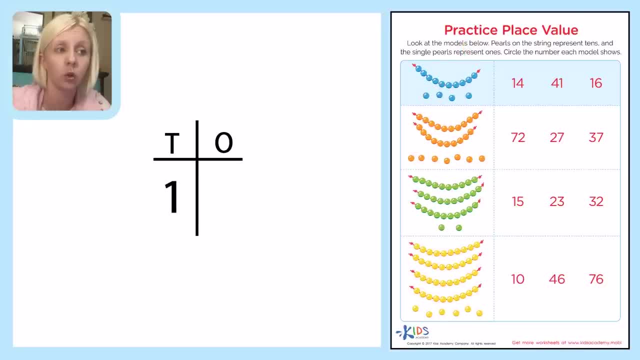 so we're going to put a one over here. and how many individual or single pearls do we have? We have one, two, three, four. So you can count those up and write it up and you can see right here we have one tens and for our ones we have four individual ones. So that's also the number 14,. 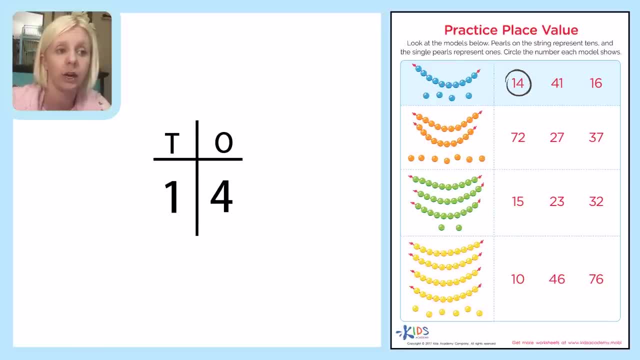 and we can come over here and we can circle it. So let's go ahead and do that. okay, Now let's go down to the next one. Let's try the next one the way that we talked about first. We're just going to count by 10.. So 10,, 20, and then, from 20, we're going to count up. 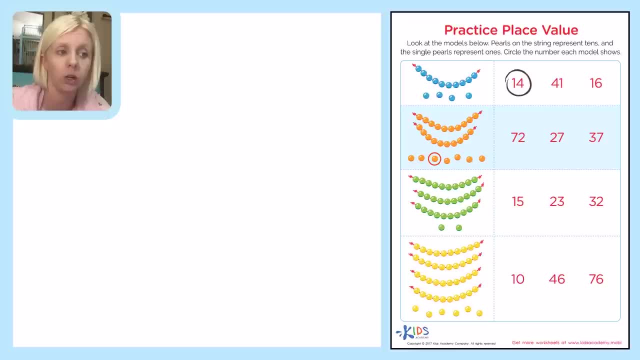 our ones. So 21,, 22,, 23,, 24,, 25,, 26,, 27.. That's kind of a fast way of doing it, and then we can come over here and we find 27, and we can circle it. The other way is to use our t-chart. okay, So we've. 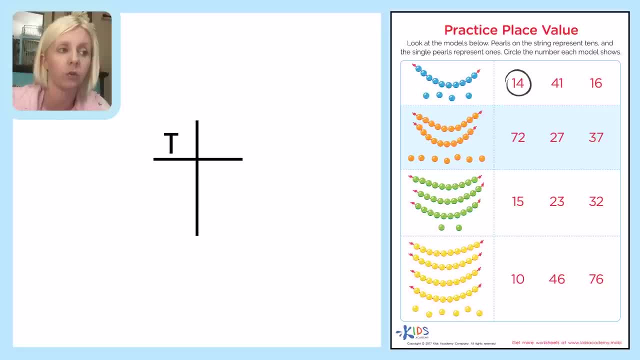 got our 10, over on this side and we've got our ones over here. So let's see how many tens do we have, or how many strings of 10 do we have. We have two, and then over here our ones One, two, three, four. 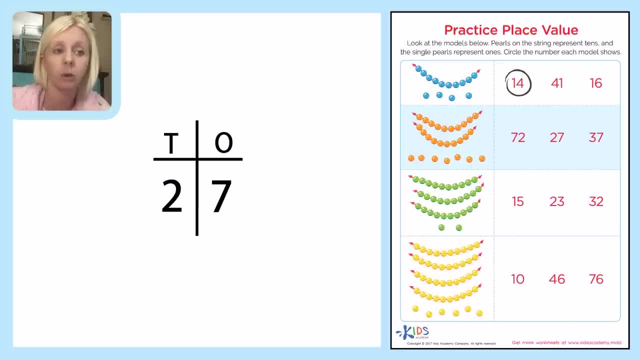 five, six, seven, So I'm going to put that right over here. and again it's the same number, It's 27.. So let's come over here and circle it. There are two ways to do it. Okay, this time let's just. 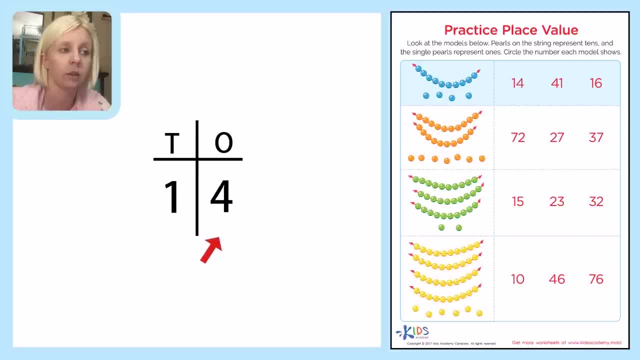 can see, right here we have one tens and for our ones we have four individual ones. so that's also the number 14 and we can come over here and we can circle it. so let's go ahead and do that. okay, now let's go down to the next one. let's try the next one the way that we talked about first. we're. 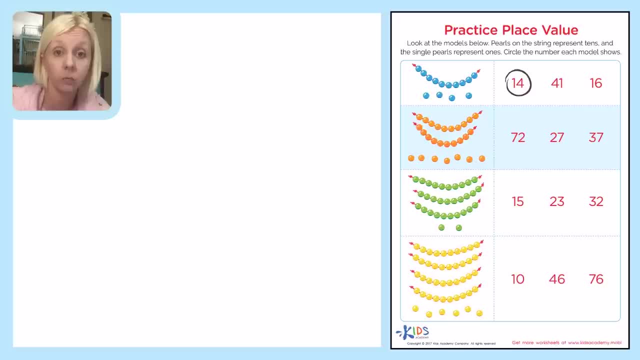 just going to count by 10, so 10, 20, and then from 20 we're going to count up our one, so 21, 22, 23, 24, 25, 26, 27- that's kind of a fast way of doing it, and then we can come over here and we find 27 and we 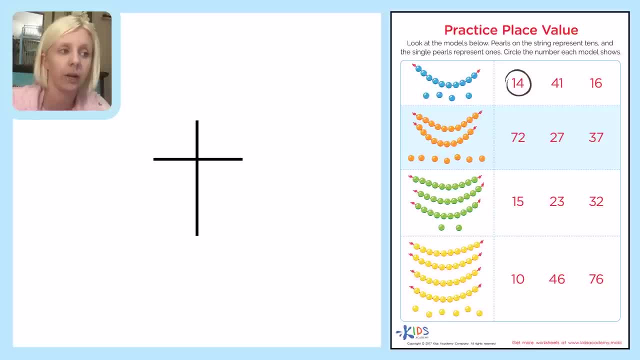 can circle it. the other way is to use our t-chart. okay, so we've got our tens over on this side and then we've got our ones over here. so let's see how many tens do we have, or how many strings of 10 do we have. we have two, and then over here our ones, one, two, three, four, five, six, seven. so I'm 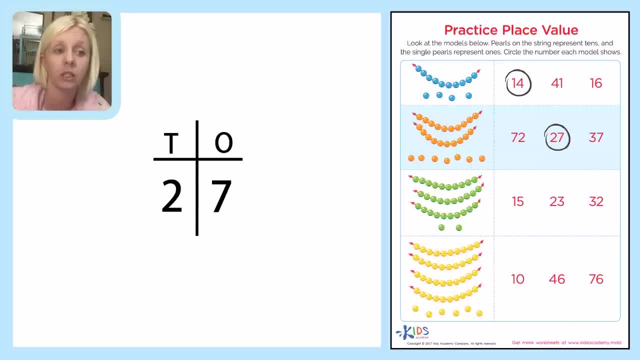 gonna put that right over here and again it's the same number, it's 27.. so let's come over here and circle it. there are two ways to do it. okay, this time let's just pick one of the ways. let's do it just by counting on. so what we're going to do is we're going to count by tens: 10, 20, 30.. 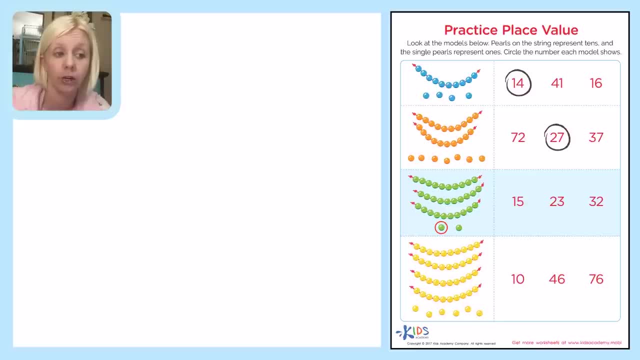 then count by 10.. count up 31, 32- okay, let's find that number 32 right over here and we're going to circle it. awesome job. and then the last one down here is our um, let's do it with our t-chart. let's do it that. 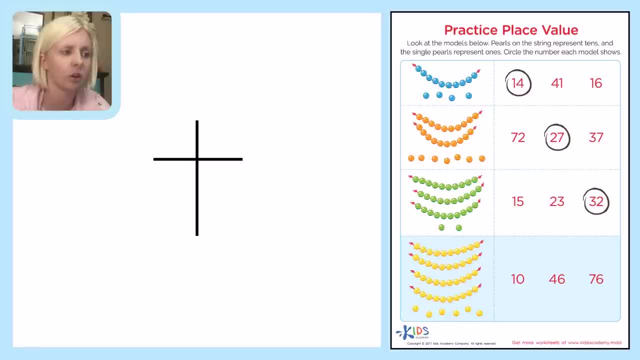 way. so let's go ahead and make up our t-chart. I like the t-chart just because it keeps everything organized, but whichever way you're comfortable with, okay, so we've got our tens place and our ones place. how many tens do we have? we've got one. 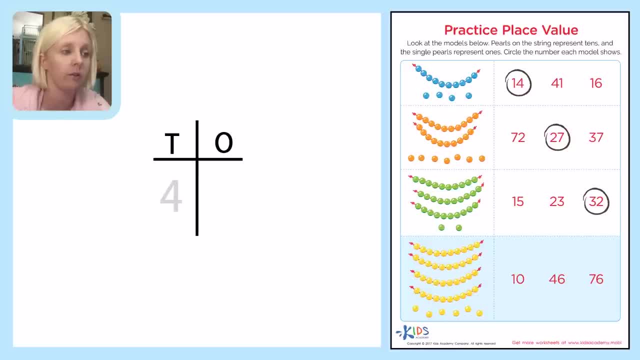 two, three, four. strings of ten. so I'm gonna put four right over here and then count our individual or our single ones: one, two, three, four, five, six. so we're gonna put our six right over here and that is the number 46.. good job, so we're gonna come over here and we're gonna circle 46. nice. 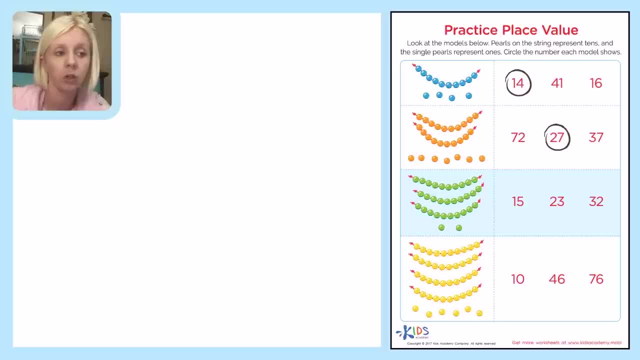 pick one of the ways. Let's do it just by counting on. So what we're going to do is we're going to count by tens: 10,, 20,, 30, then count up 31,, 32.. Let's find that number 32 right over here and we're going to circle it. 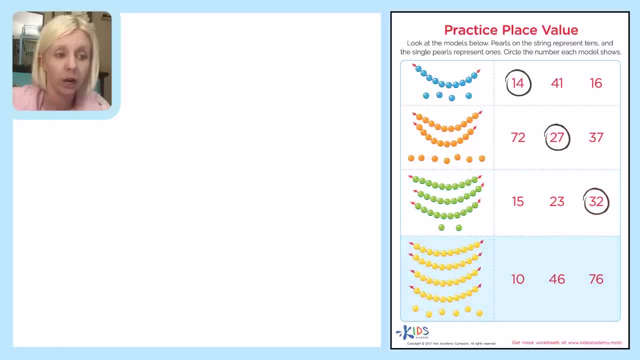 Awesome job. And then the last one down here is our: let's do it with our t-chart. Let's do it that way, So let's go ahead and make up our t-chart. I like the t-chart just because it keeps everything organized. 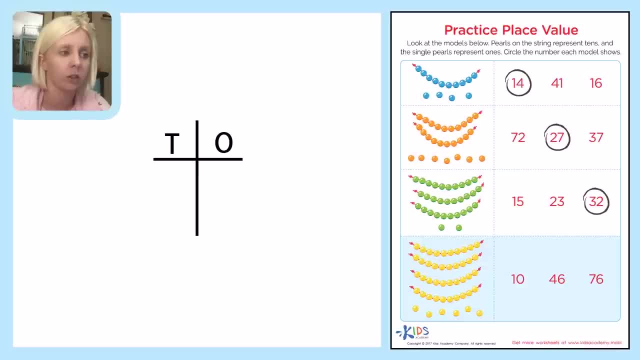 but whichever way you're comfortable with. So we've got our tens placed and our ones placed. How many tens do we have? We've got one, two, three, four strings of ten. So I'm going to put four right over here And then count our individual or our single ones: One, two, three, four, five, six. 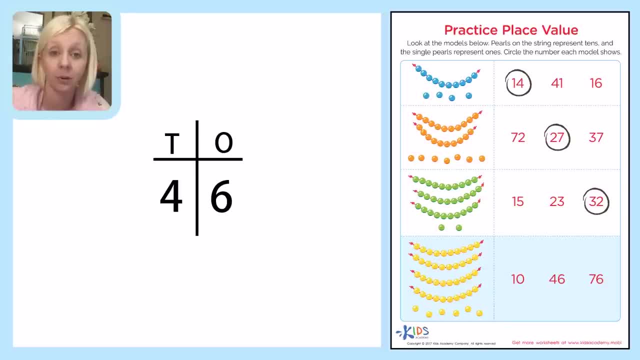 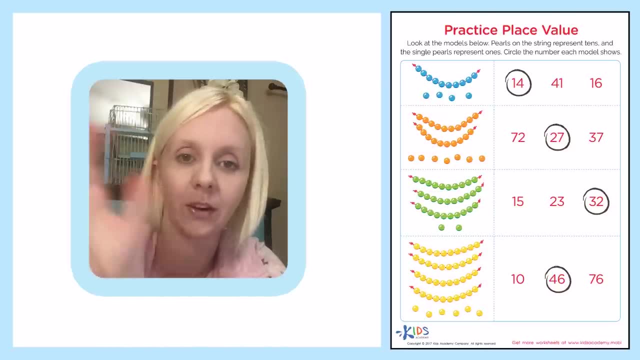 So we're going to put our six right over here And that is the number 46.. Good job, So we're going to come over here and we're going to circle 46.. Nice job today with your place value. Bye-bye. 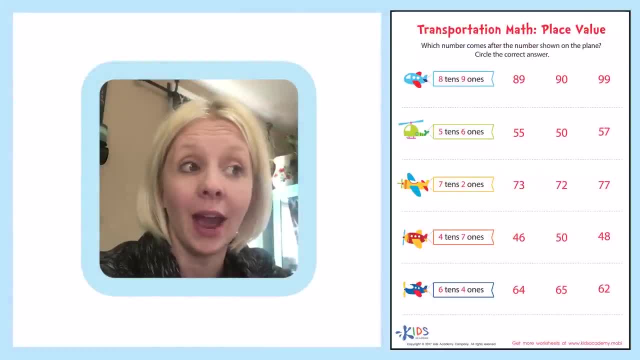 All right. So we have the worksheet named Transportation Math Place Value. Which number comes after the number shown on the plane Circle, the correct answer. So what we're going to do is we're looking at these different numbers here And we've got this first number, Our first number. 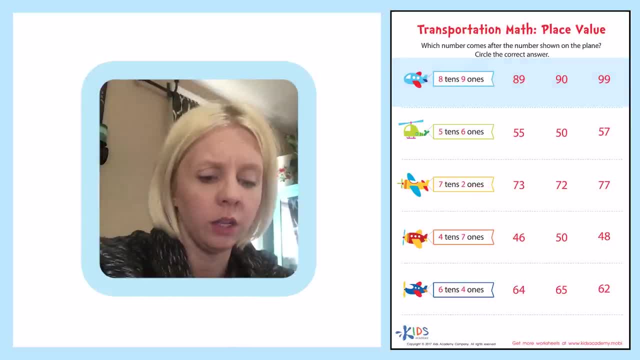 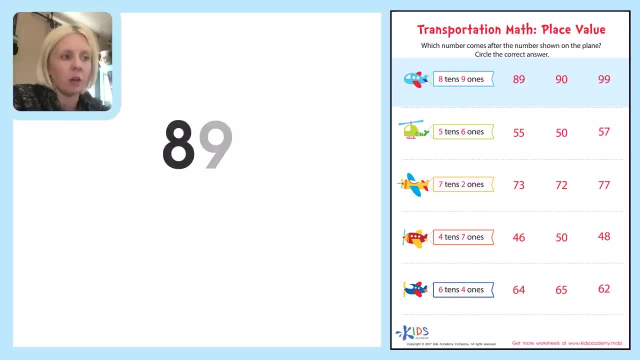 is 810s and 91s. Let's write that number out to the side over here We've got 810s, 10's and 9 1's. Okay, so that is the number 89.. The question says which number comes after the. 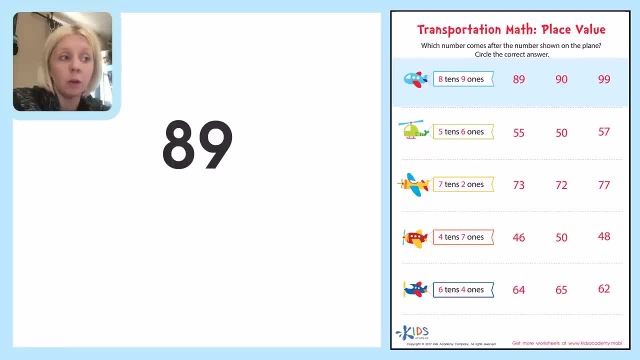 number shown on the plane. So if we were counting, what would be the number that would come after 89?? Well, normally we're just looking at the 1's place and the 1's will change. But when we come to 9, we don't go to 10. We actually go to 0 and then the 10's place moves up 1.. So the next number. 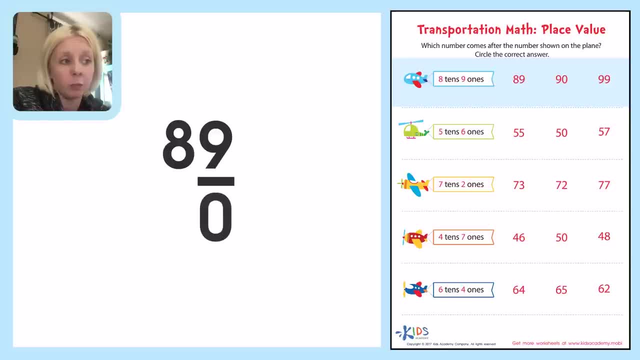 we would put 0 after the 9, and then the 10's place would move up 1,, which would be 9.. Okay, so our next number is 9.. 89, 90.. That's our next number. So we're going to come over here. 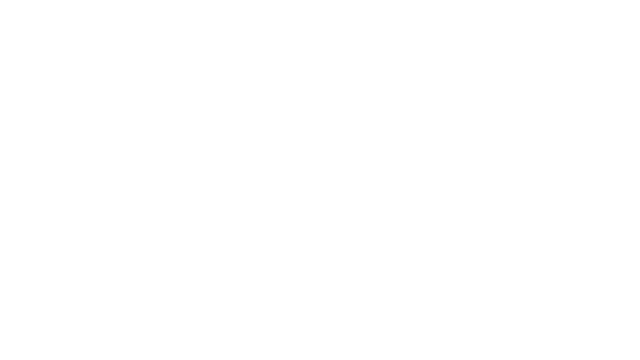 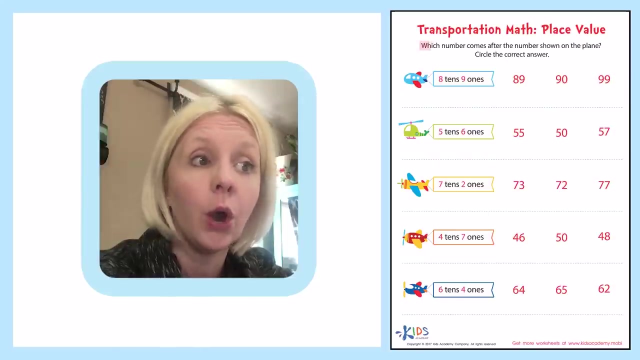 job today with your place value, bye-bye. all right, so we have the worksheet named notation math: place value. which number comes after the number shown on the plane circle? the correct answer. so what we're going to do is we're looking at these different numbers here and we've 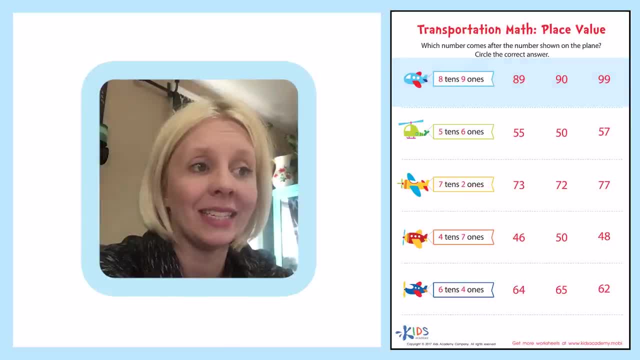 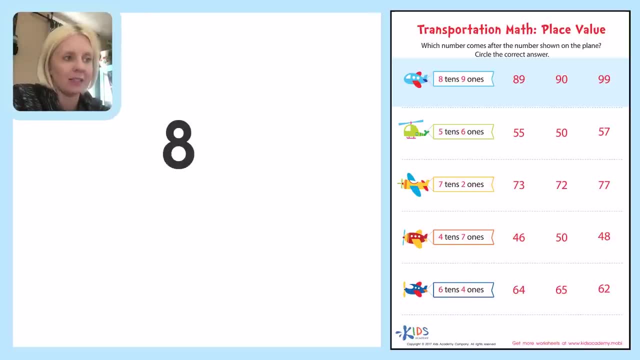 got this first number. our first number is eight tens and nine ones. let's write that number out to the side over here. we've got eight tens and nine ones. okay, so that is the number 89. the question says which number comes after the number shown on the plane. so if we were counting, 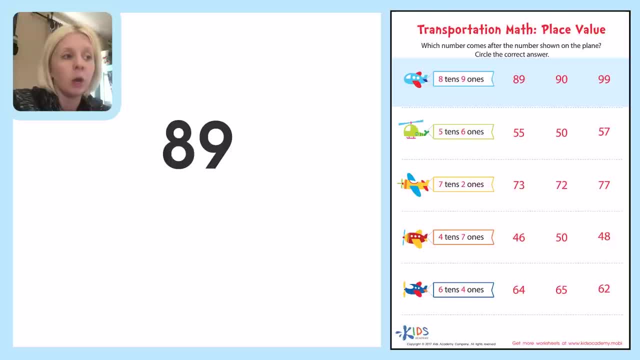 what would be the number that would come after 89.. well, normally we're just looking at the ones place and the ones will change. but when we come to nine, we don't go to ten, we actually go to zero, and then the tens place moves up one. so the next number, we would put zero after the nine, and then 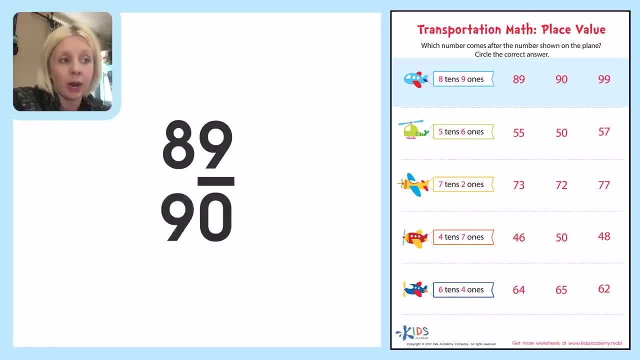 place would move up one which would be nine. okay, so our next number is 989 90. that's our next number. so we're going to come over here and we're going to circle it, okay, the next one is five tens and six ones, that's the number 56, and I told. 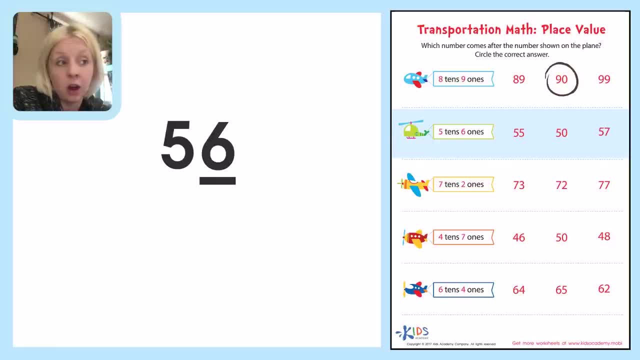 you, normally we're looking at the ones place. as long as it's not a nine, then it's just going to be the number right after it. so what comes after six? the answer is seven. the five stays the same, so our answer is going to be 57, so come? 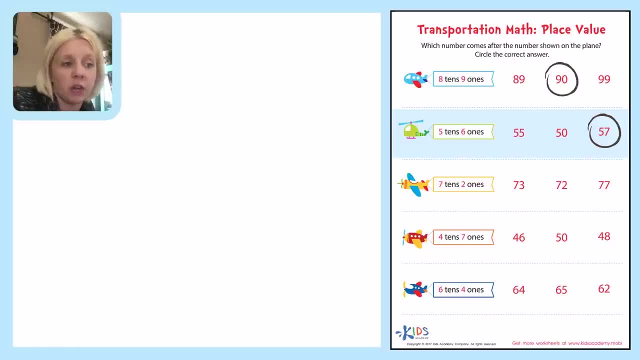 right over here we're going to circle 57, 56, 57- that was our next number. okay, the next one is seven tens and two ones. okay, so we're gonna find the number right after two is going to be three. seven stays the same, so we've got 73, that's. 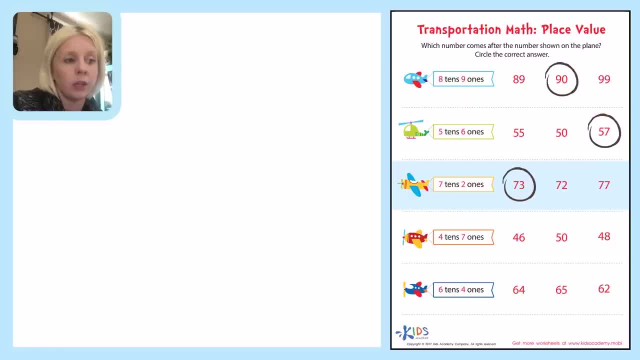 our next number, we're gonna come right over here and we're going to say: circle it. the next one is four tens and seven ones, and we're just looking at the ones place seven. what comes after seven is eight. our four stays the same, so 47. 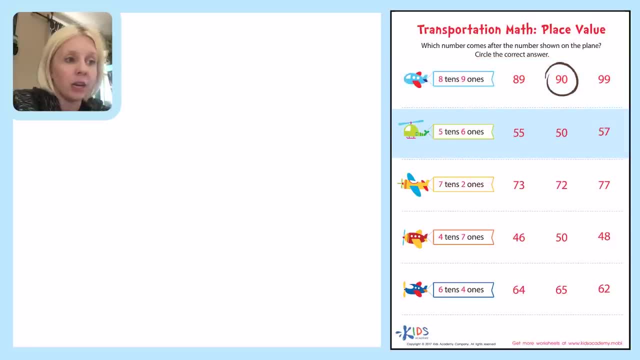 and we're going to circle it. Okay, the next one is 5 10's and 6 1's. That's the number 5.. 56. And I told you, normally we're looking at the 1's place As long as it's not a 9,. 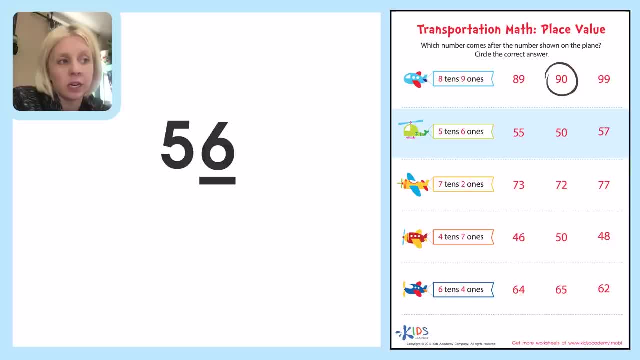 then it's just going to be the number right after it. So what comes after 6?? The answer is 7.. The 5 stays the same, So our answer is going to be 57.. So come right over here, We're going to circle. 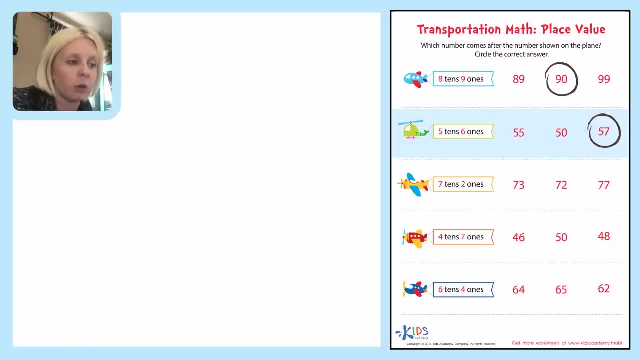 57.. 56, 57.. That was our next number. Okay, the next one is 7 10's and 2 1's. Okay, so we're going to find the number. So we're going to find the number. So we're going to find the number So. 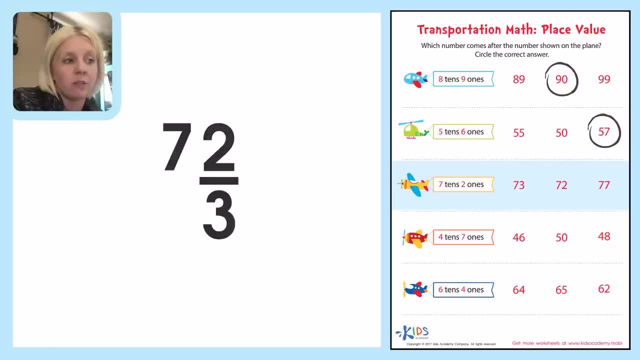 the number right after 2 is going to be 3.. 7 stays the same, So we've got 73.. That's our next number. We're going to come right over here and we're going to circle it. The next one is 4- 10's and 7- 1's, And we're just looking at the 1's place, 7, what comes after 7 is 8.. Our 4 stays the same, So 47, 48.. Okay, and I'm going to circle that right over here. Great job. 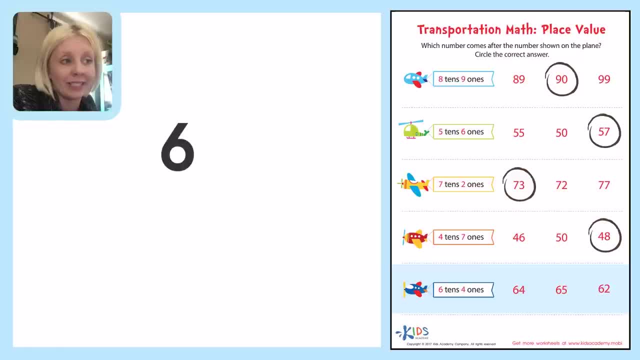 We've got one more. The last one says 6 10's and 4 1's. Okay, so we're going to look right here What comes after 4? 5.. Our 6 stays the same, So it's 64, 65.. Okay, great job. Bye. 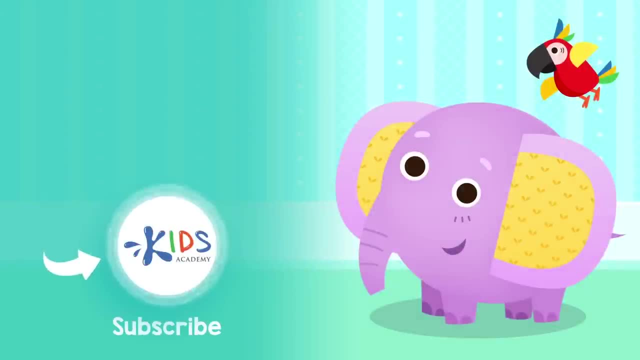 Subscribe to our channel to stay updated on new videos. Find links to our apps in the comments below.